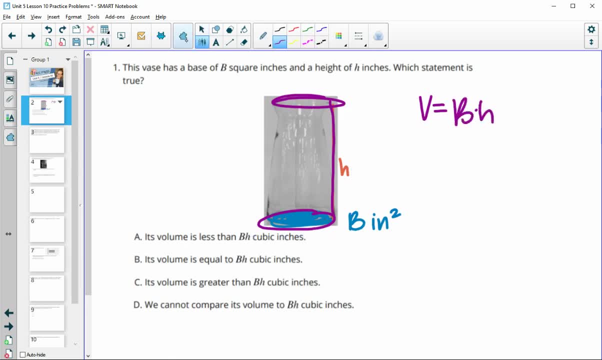 the area would be area of the base times the height. Now, with this problem we're going to take a look at the Unit 5, Lesson 10, Practice Problems. So this one, it doesn't just go directly up to the top, It kind of cuts in here and this looks to be smaller than this blue base. 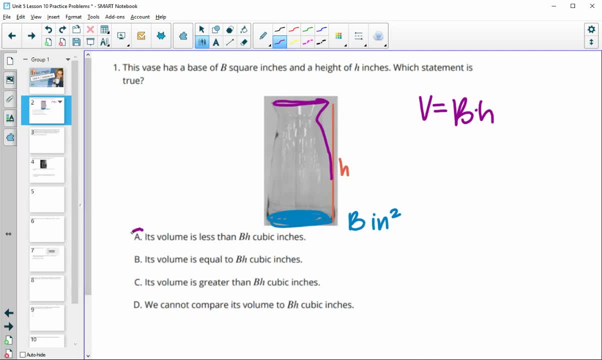 So the volume of the actual vase is going to be less than just the area of the base times the height. So it's not going to be equal to it because it's not uniform. It's not going to be greater than because it goes back in and we definitely can compare it to those. 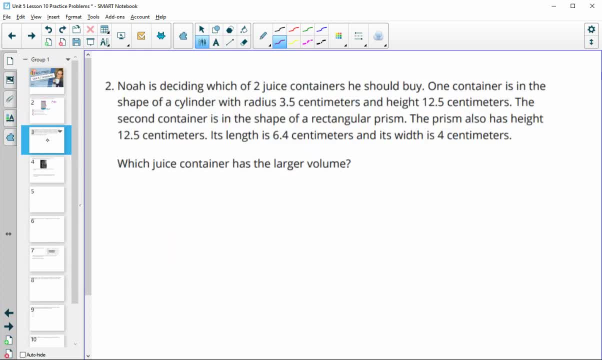 So A would be That's going to be the correct answer there. All right, And number two: Noah's deciding which of two juice containers he should buy. One container is the shape of a cylinder and then the other is the shape of a rectangular prism. 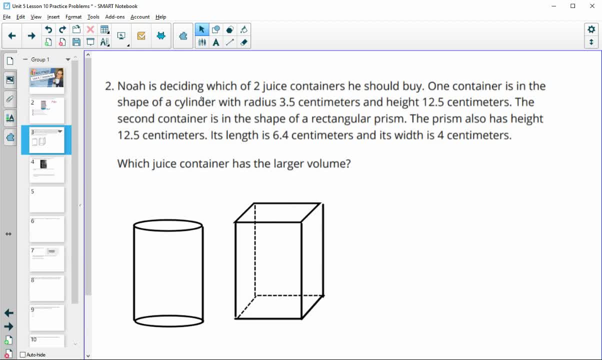 Okay. So then it says the shape of the cylinder has a. the one that's the shape of a cylinder- The one that's the shape of a cylinder- has a radius of 3.5 centimeters and then a height of 12.5 centimeters. and then it says the rectangular prism also has a height of 12.5 centimeters, and this one has a length of 6.4 and a width of 4.. 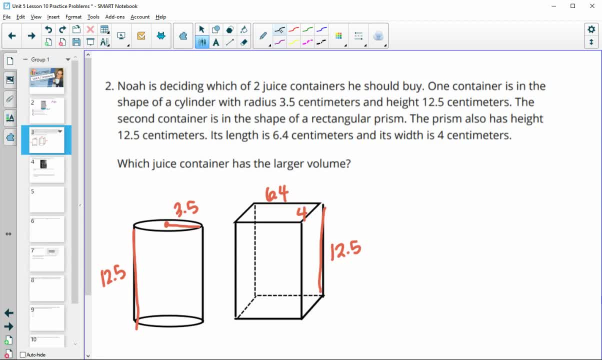 So which juice container has a larger volume? So remember, for volume it equals area, The area of the base times the height, But in this case the heights are exactly the same. So whichever of these two shapes has a larger base area will have a larger volume and therefore be a better deal, as long as they're the same cost. 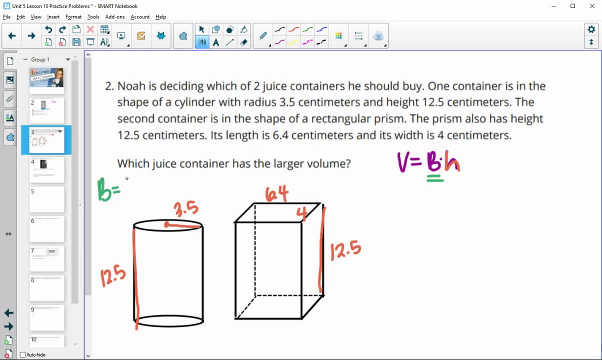 So for this cylinder the area of our base is going to be 3.5 squared times pi. And so If we multiply that out to get an actual decimal version, we would get 38.48 centimeters squared. And then for this one, if we do 6.4 times 4, we will get a base area of 25.6.. 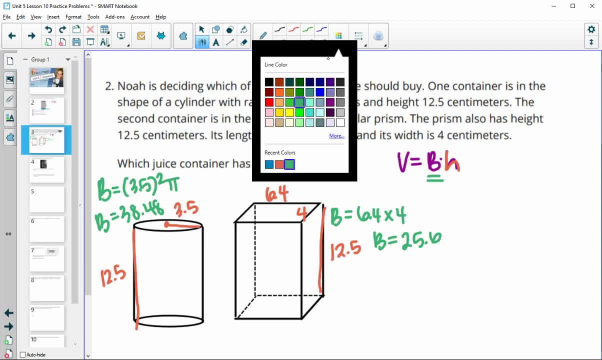 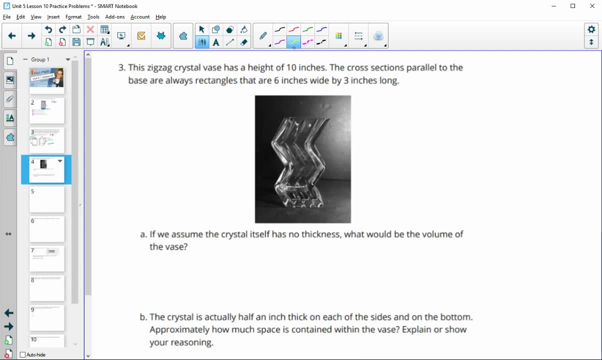 So the cylinder is going to have the larger volume because it has The larger base area and they have the exact same height. So it's going to be the cylinder in this case. Number three, this zigzag crystal vase has a height of 10 inches. 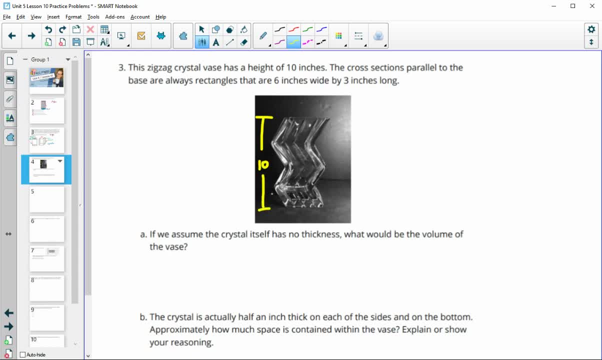 So this is 10 inches and the cross sections parallel to the base are rectangles. OK, so you kind of get rectangles here that are six by six by three. So this says, if we assume that the crystal has no thickness, what would the volume of this vase be? 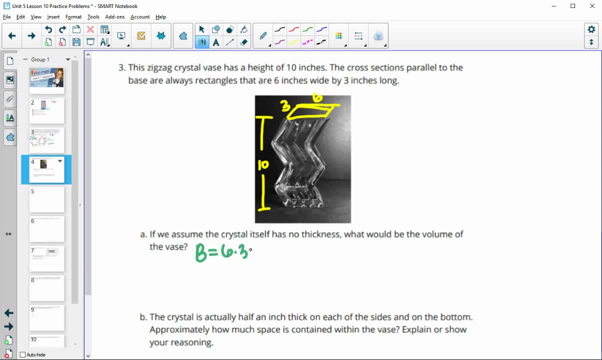 So we would be doing area of the base which is six times three or 18, and we would be multiplying that by the height, So the volume would be 18 times 10 or 180 inches cubed. So that would be if that crystal was just supersized. 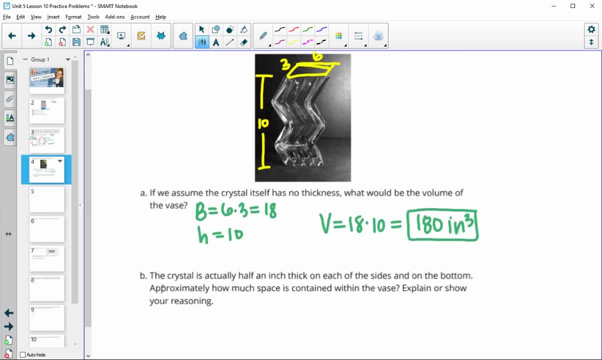 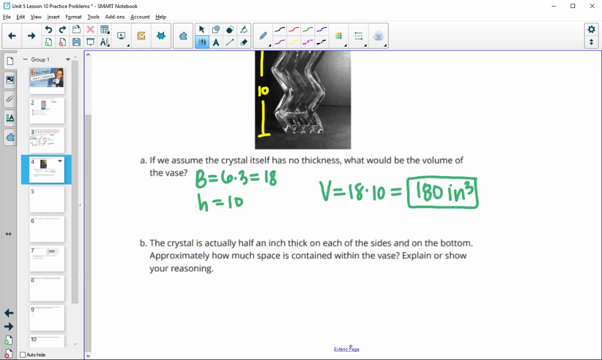 So that would be if that crystal was just super thin and didn't have any width. Now, if the crystal is actually one half inch thick on each of the sides and on the bottom, approximately how much volume would this one have? And so when we do this, this is going to take in some of our dimensions. 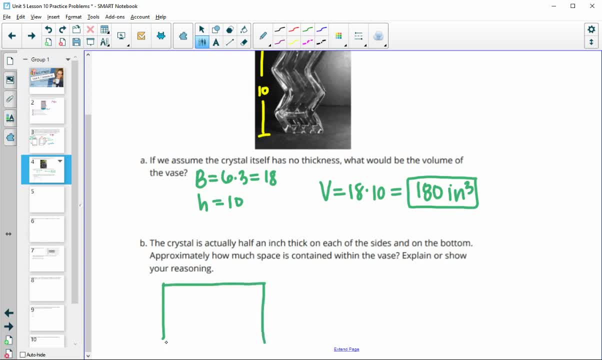 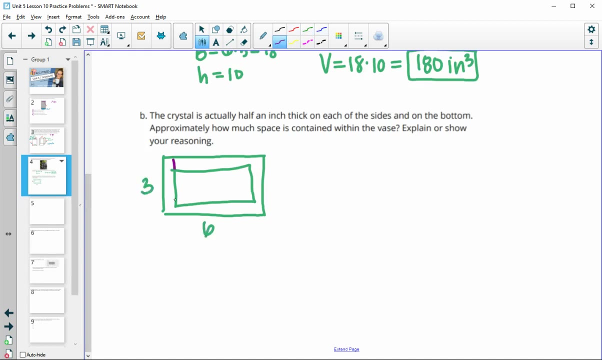 So now we had this rectangular base here And this rectangular base This is now in a half inch, with glass on each side. So before it was six by three, Now you've got a half inch taken in on both sides here, So this is actually two inches and you have a half inch taken in here. 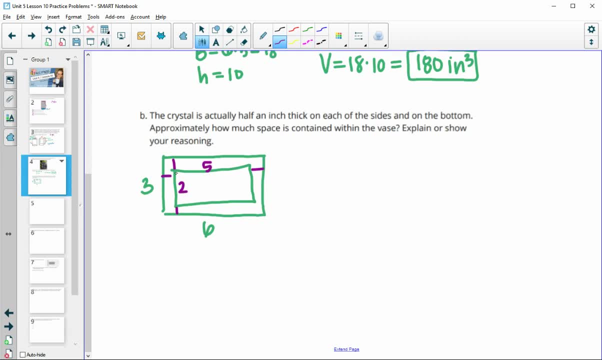 So that's one full inch, So that's going to be five. So this inner, this inner rectangle here, is actually a two by five rectangle, Or 10 for that base Now, when you think about the height. so that's your base area. 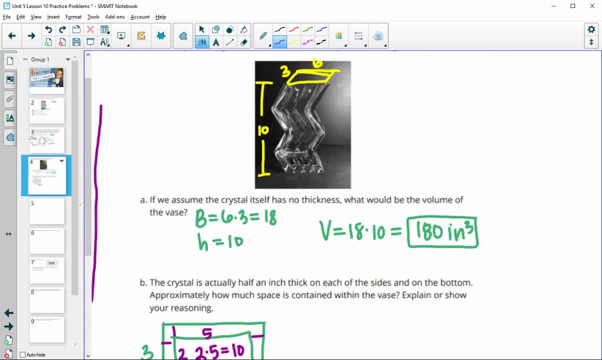 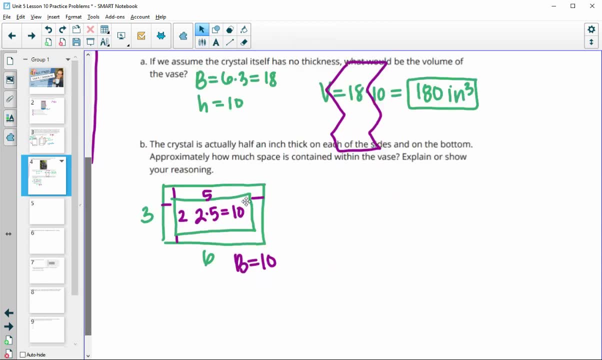 Now when we think of the height of this base, So if I just kind of redraw this base and take it down here, So now when we're talking about the height, now part of your height is taken in by a half inch thick glass from top to bottom. 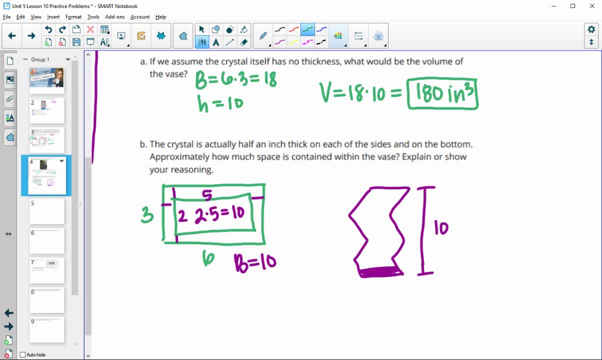 So where this used to be 10, now with this half inch here, okay, that new height is going to be 9.5.. So when we do the volume, we're going to be doing 10 times 9.5, which is going to give us 95 inches cubed if we have to take in on each side there. 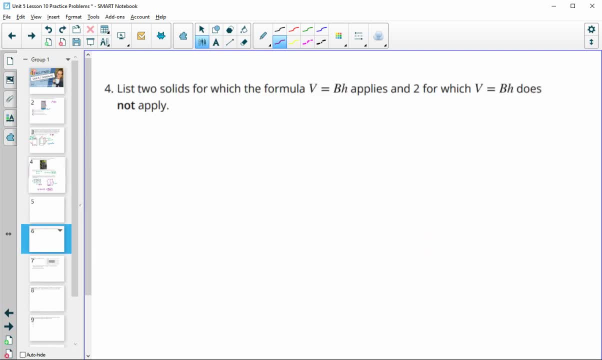 All right, then number four, List two solids for which the formula volume equals area of the base times height applies, and two for which it doesn't. So we've done a couple. We did a cylinder And a rectangular prism, So those are two that it would work for. 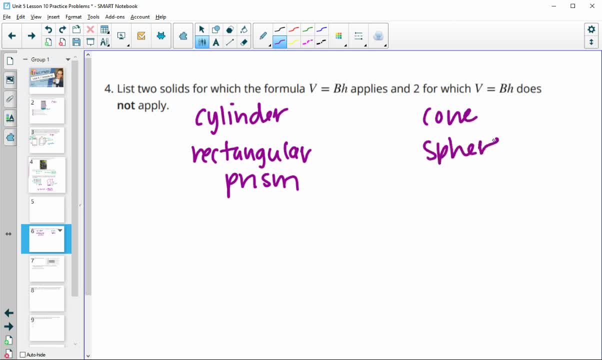 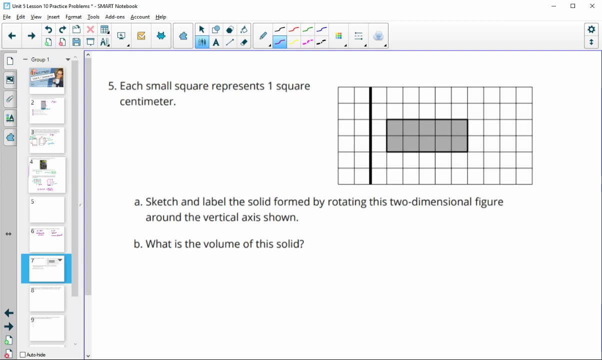 So a cone wouldn't work, A sphere wouldn't work. Those are two examples You could do. any type of pyramid Wouldn't work. Number five: Each small square represents one square centimeter. Sketch and label the solid form by rotating this figure around the vertical axis. 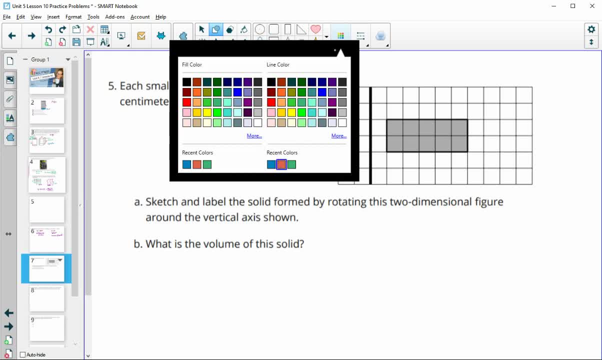 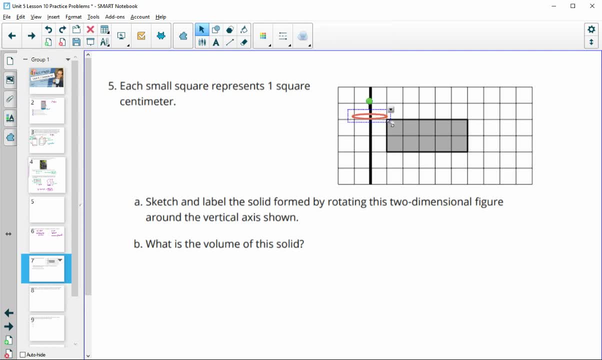 So I'm just going to use these circles to draw it So we'd have kind of this hole in the middle right that has a radius of one. Then we would also have a circle formed, kind of this big, that goes that full distance on top and bottom. 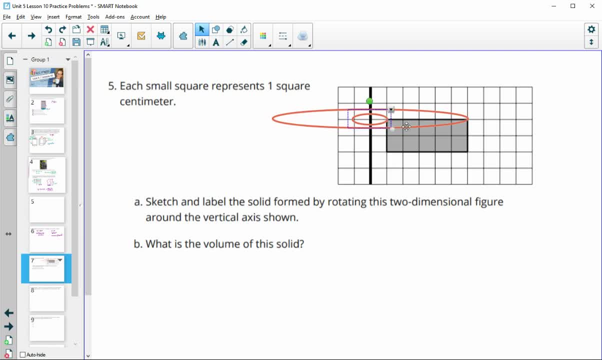 We would have this And then the height kind of between these would be two, which is the height of this Two-dimensional thing here. So let me get this in And that would go here. It would also connect these inner circles as well. 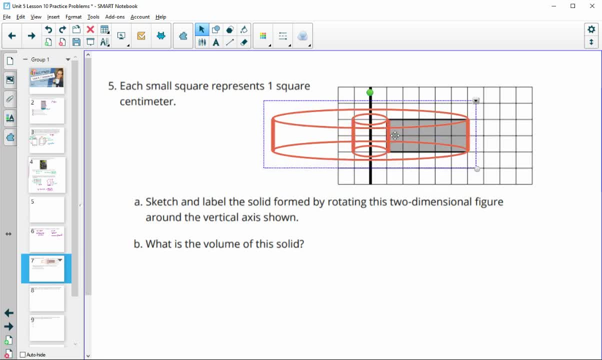 And so this would be a sketch of the three-dimensional solid, And now this inner part is Hollow, And then the rest of it would be filled in. So then let's figure out the volume here. So this inner hollow part has a radius of one. 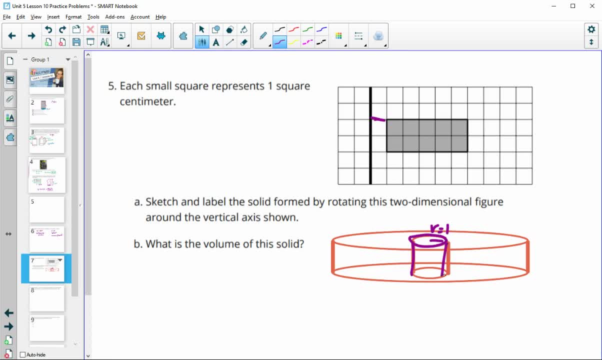 So if we were going to find the area or, sorry, the volume of this, Okay, then the height is two, So the volume would be the area of the base, And the area of this base would be one squared times pi for that circle. 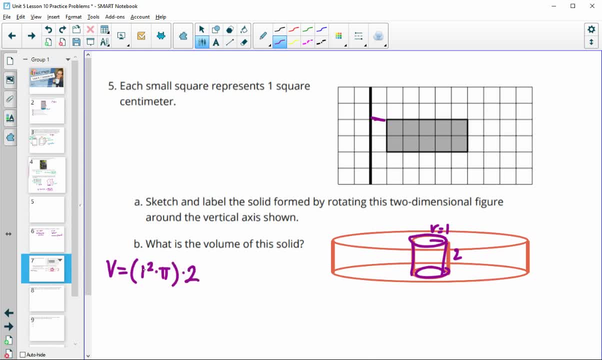 And then times its height, which is two. So one squared is one times two. So the volume of that inner cylinder is two pi. Then we would want to find the volume of the larger cylinder, And so now, going all the way into the middle here, that's going to be one, two, three, four, five, six for the radius. 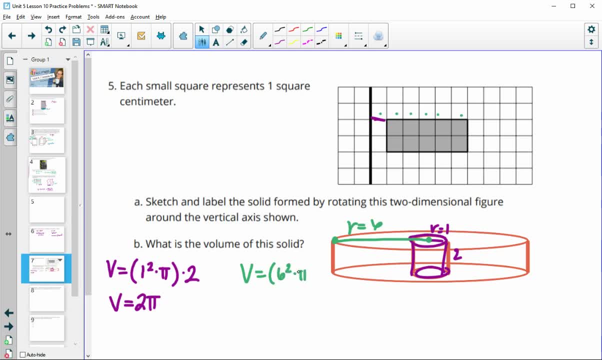 So the area of this base is going to be six squared times pi, And then we're going to multiply by the height, Okay, Which the height of this is still two, And so we'll do six pi, or six squared pi, times two. 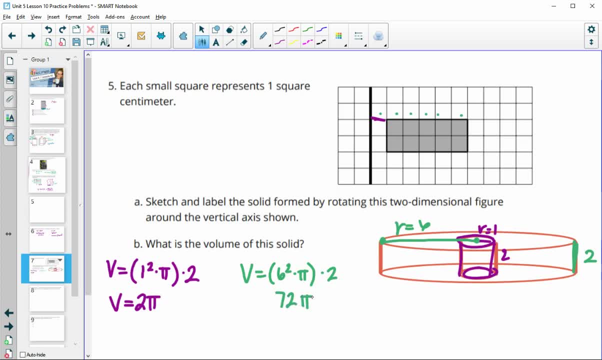 So this is 36 times two, would be 72 pi for the volume of that larger cylinder And then we would just subtract that inner volume And that would give us our total volume of 70 pi, And then centimeters cubed. Okay. 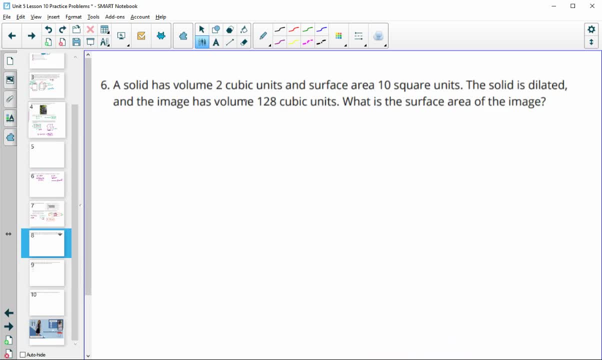 Number six, a solid has a volume of two cubic units. It has a surface area of 10 square units And then it has a volume of 128. And the original volume was two. What is this new surface area? So they gave us both volumes. 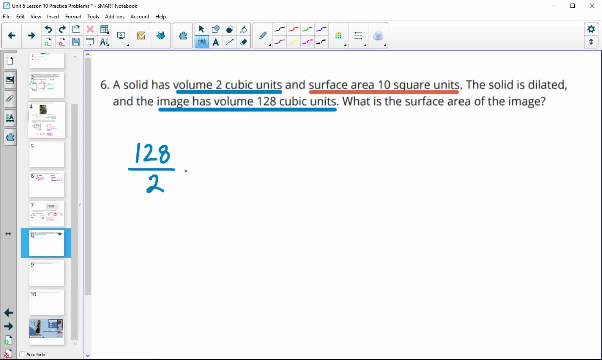 So we'll compare the new volume to the original volume And when we compare volumes that gets us our scale factor cubed. So then 128 divided by 2 is 64 for K cubed. That will help us get the scale factor by cube rooting this. 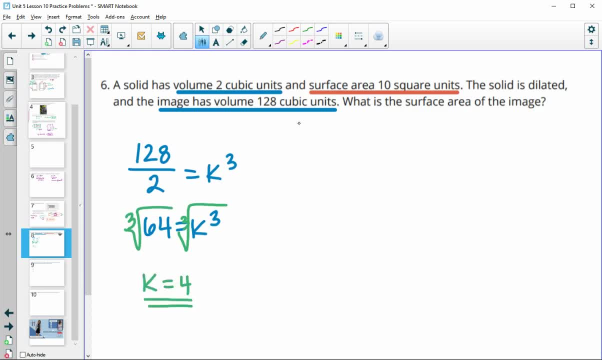 And the cube root of 64 is 4.. So our scale factor is 4.. So then when we have the area, we will do the area times the scale factor squared to get our new area. So our original area here is 10.. 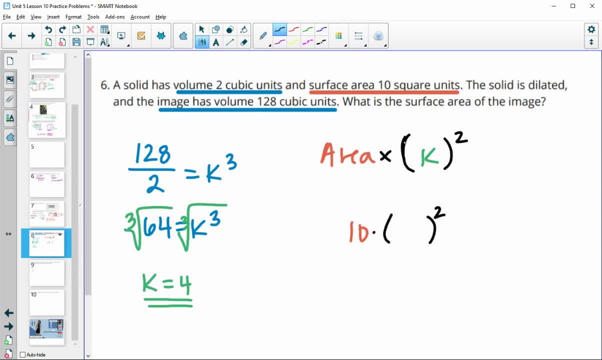 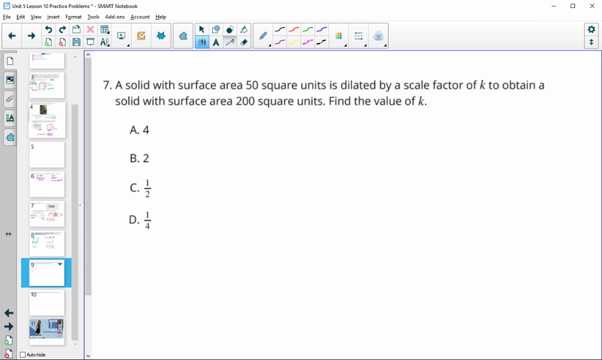 So we will multiply that by 4 squared, So we're doing 10 times 16.. So our new area is going to be 160.. Units squared Number 7.. So we have a solid that has a surface area of 50 units squared. 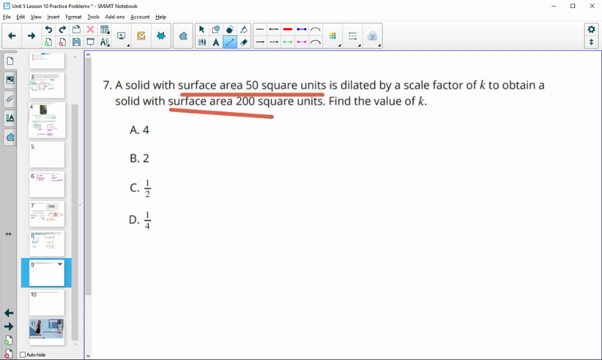 It's dilated by some scale factor, to get a new surface area of 200.. What's the scale factor? So when we compare areas- new area to original area- we're going to get a new surface area of 200.. So we're going to get our K squared value. 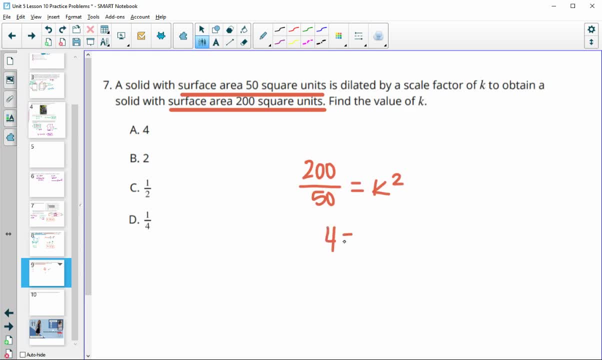 So 200 divided by 50 is 4.. So this is our K squared. So to get our scale factor, we are going to square root both of those And we would get a scale factor of 2. Number 8.. Number 8.. 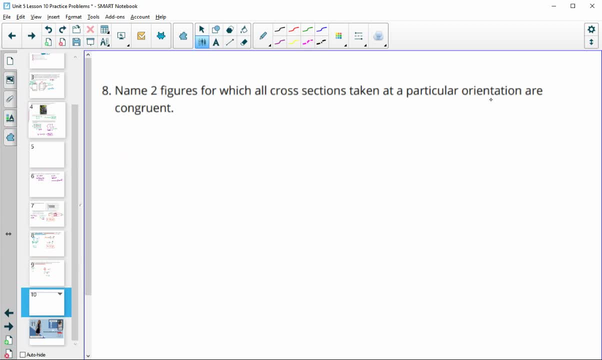 Name two figures for which all cross sections taken at a particular orientation are congruent. So we would want to make sure that this isn't changing its size at all. So we could do any type of prism, So if we did like a square or a rectangular prism, 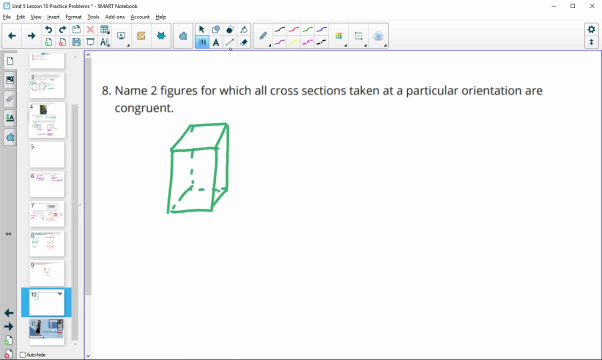 and then we said we were going to do the cross section, the horizontal cross section. So if we were going to be looking at a horizontal cross section here, it would stay the same all the way up, Because you'd end up with this: 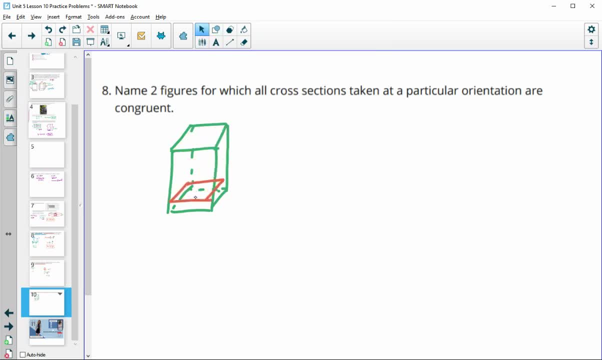 And then this would be the same cross section from top to bottom. Or even if you did a vertical cross section, this would stay the same vertically all across the shape. So a prism, really any type of prism, So you could also do a triangular prism. 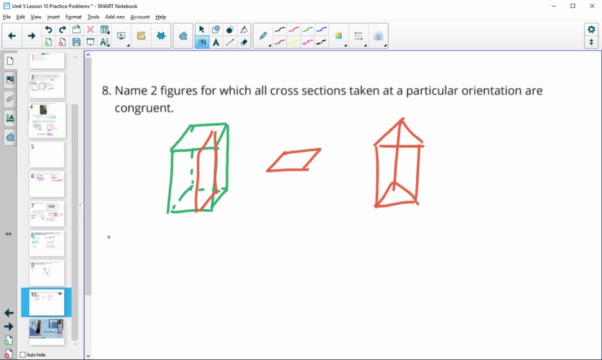 and that would be the same as well. Number 9..